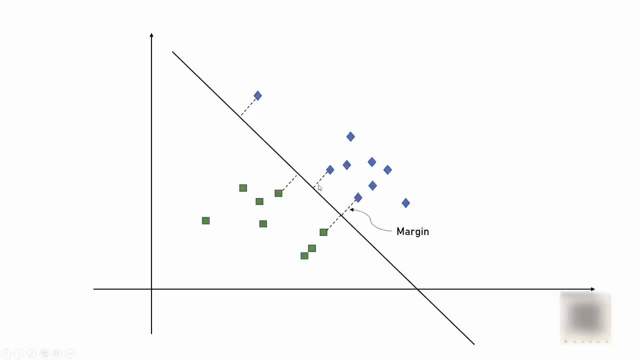 will try to maximize this margin here between the nearby data points and the line itself. and these nearby data points are called support vectors, hence the name support vector machine. so in case of a 2d space where you have two features, the boundary is a line. in case of 3d, the boundary is a plane. what will? 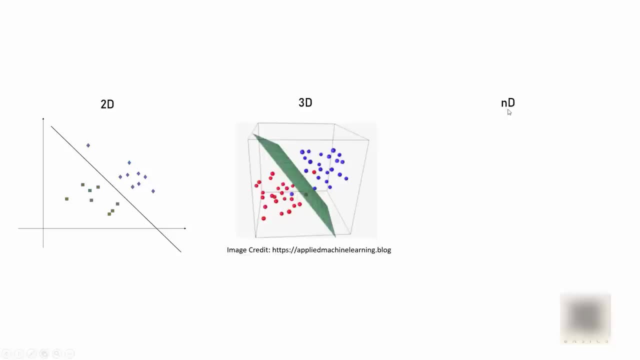 it be. if you have n dimensional space, usually you have n number of features, right? so just pause this video for a moment. try to visualize what that boundary will look like, and you will realize that it's kind of impossible to visualize it, but theoretically or mathematically. 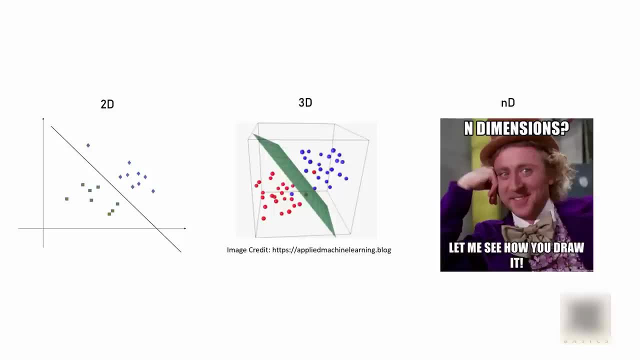 it's kind of impossible to visualize it, but theoretically or mathematically it's still possible and that boundary is called a hyper plane. so hyper plane is a plane in n dimensional and dimension that tries to separate out different classification groups, and that's what support vector machine algorithms tries. 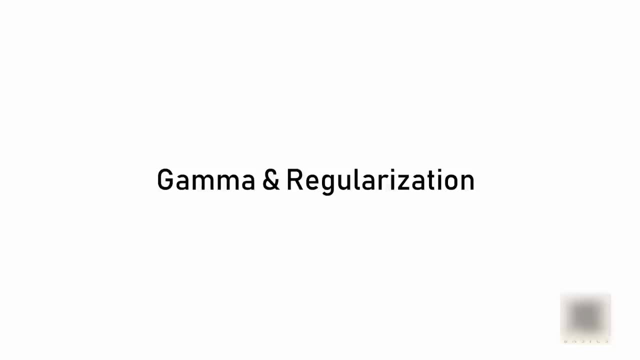 to do so, we need to familiarize ourselves with certain technical terms, such as gamma and regularization, and we'll go over these terms. so on this graph, you can see that this decision boundary is only considering the data points which are very near to it. okay, so this is one way of drawing a decision boundary. you 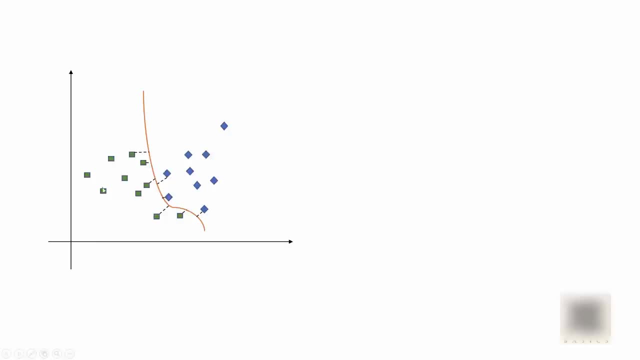 can see that I have excluded these data points and these far away data points in making my decision for the decision boundary. the other approach of looking at same problem could be that you consider the far away data points as well. so on the left-hand side I have a high gamma and right-hand side I have a 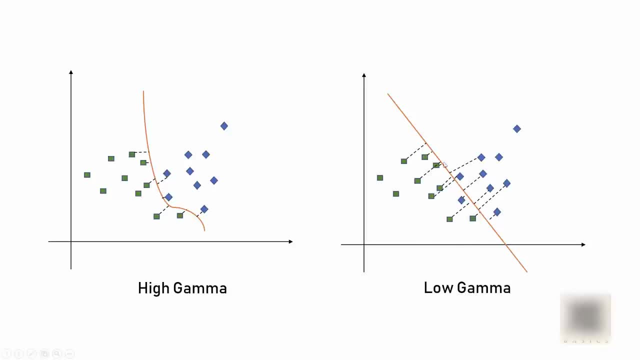 low gamma and both the approaches are valid. it's just that with low gamma sometimes you might get- you might get accurate problem with accuracy but that might be okay. you know it might be computationally more efficient. so both the approaches are right. it depends on your individual situation. the other 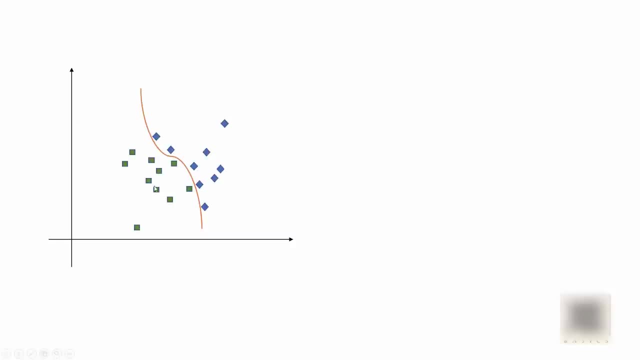 example here is: this is a separate data set where I try to draw my boundary very carefully to avoid any classification error. you can see that this is almost overfitting the model. so if you have a very complex data set, this line might be- might be very. 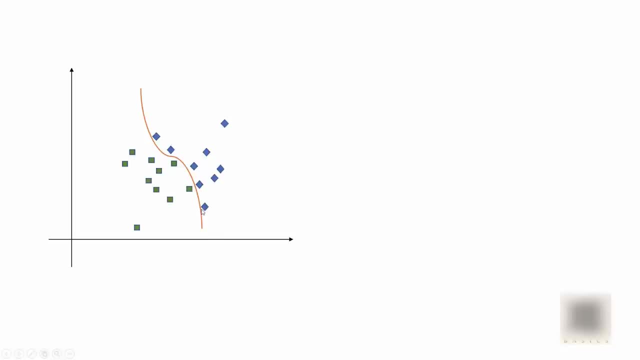 zigzag and wiggly and it might try to overfit the model. on the other hand, I can take some errors. so here you can see that I have a very complex data set and you can see that there is this classification error which might be okay. 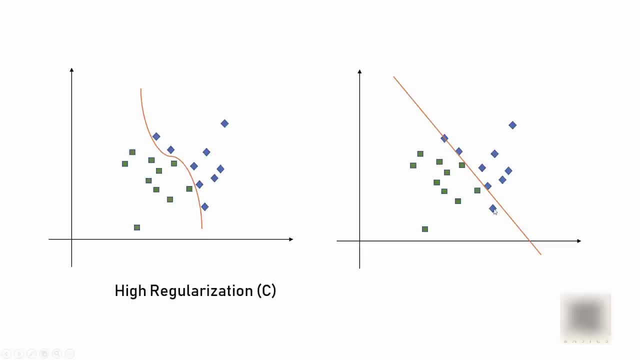 and my line might look more smoother. so on the left-hand side what I have is a higher regularization. on the right hand side, I have a low regularization. with low regularization you might get some error, but that might be okay. that might be even better for your model when we'll use sklearn library to train our model. 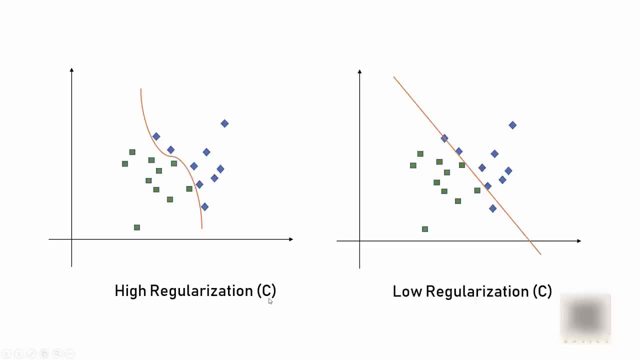 you will see a parameter called C, and C means głos regularization. basically, you might have a complex data set like this. so what do you do like here? it's not very easy to draw the boundary. one approach is create a third dimension. so I have X and Y here. so what if you create Z dimension and 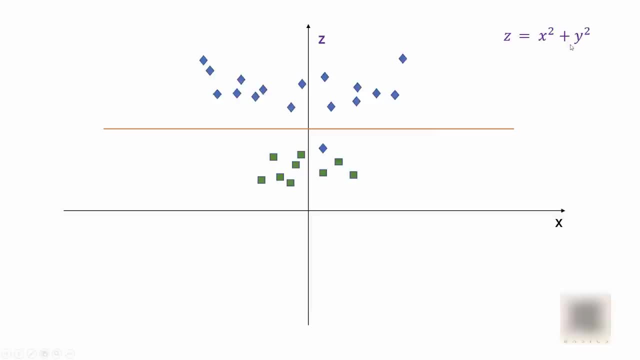 the way you do it, by doing x square plus y square, so you are doing some transformation on your basic features and creating this new feature here, and with that you will be able to draw this decision boundary. so the Y plane is perpendicular to your monitor right now, so that's why you are not able to see it. 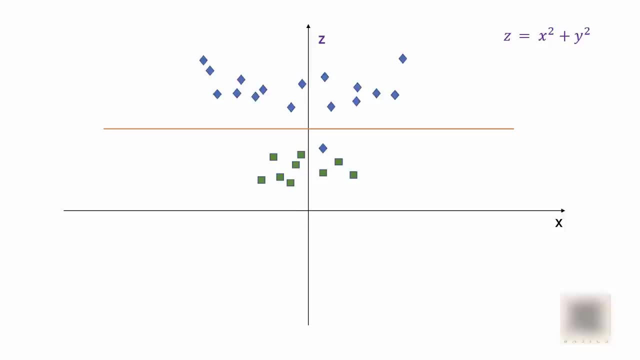 okay, so just try to visualize the situation. it's not very hard. and once you have the boundary, you can superimpose it on your Y plane, Y and X, the plane formed by X and Y axis, and you will get a boundary like this. so the Z here is called a kernel by kernel, what we mean. 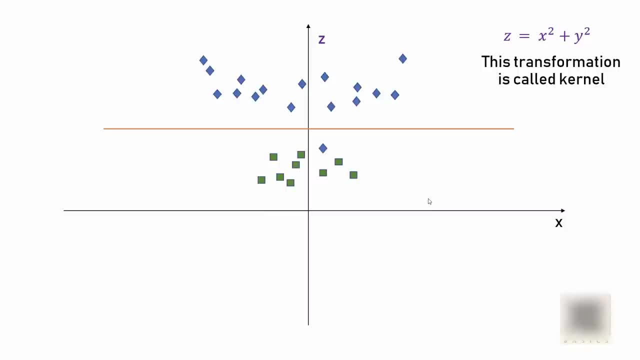 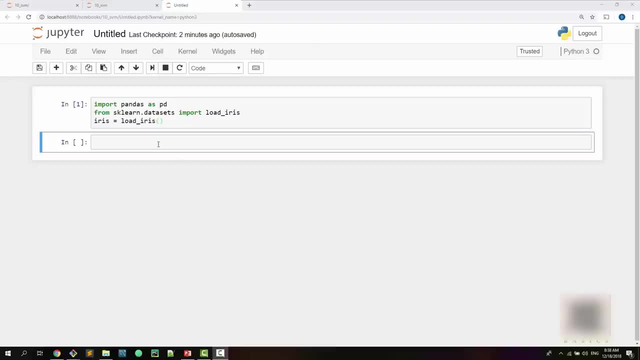 is, we are creating a transformation on your existing features so that we can draw the decision boundary easily. as usual, I have my Jupyter notebook open here and I have imported iris data set from a scale on library and when you look at the iris data set- the basic features you will see it has these: 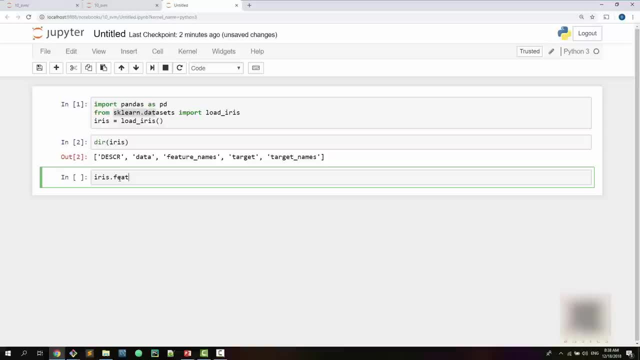 values. right, and when I do feature names, I'll see the four features that I shown. you showed you in the first picture. alright, so what I'm going to do is create a data frame out of this, because it's easier to visualize this data set with a data frame, so I will do something like. DF is equal to PD. 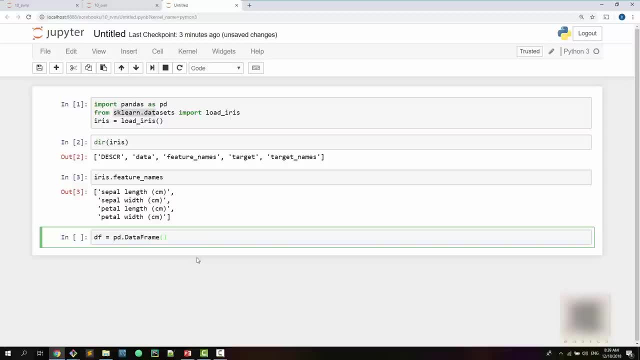 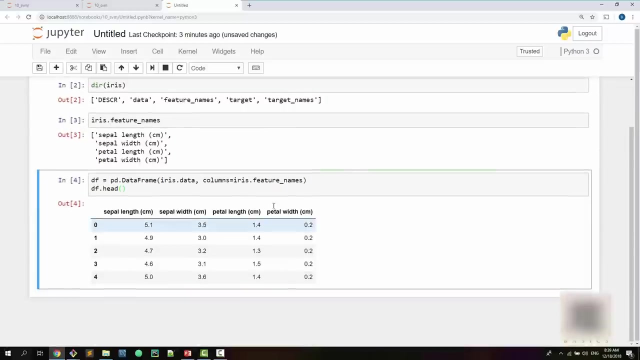 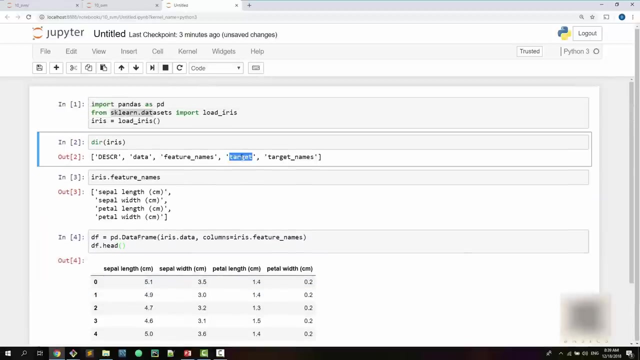 dot data frame and my data is in this iris dot data and my columns is actually the feature names. all right, and when you do DF dot head, you will see that I have a nice data frame like this ready. I also have target wave table in this target parameter so I will append one more column called target in. 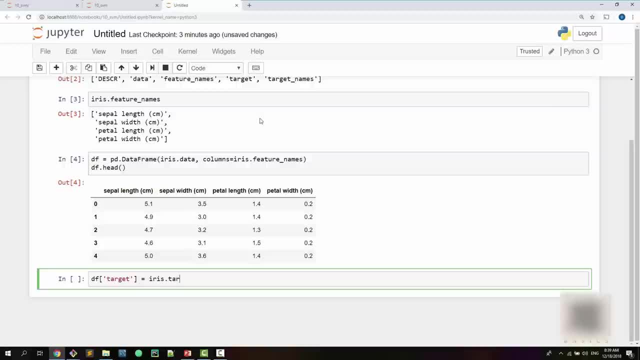 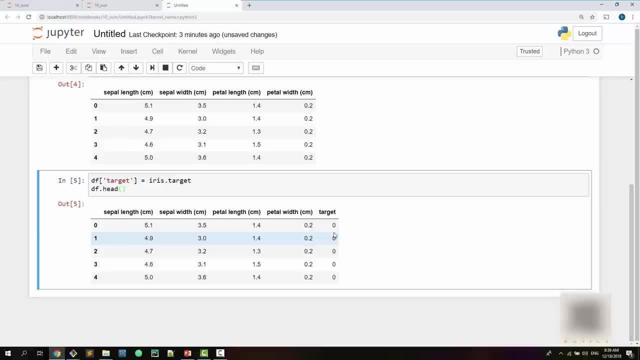 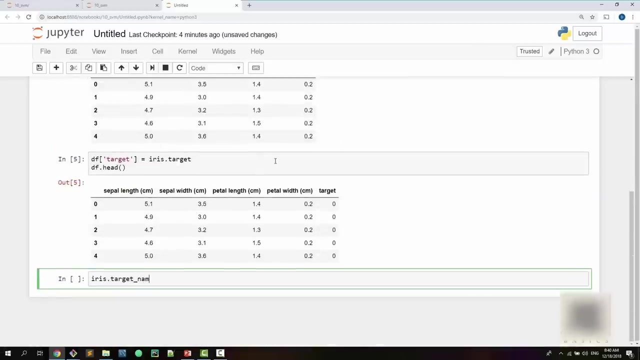 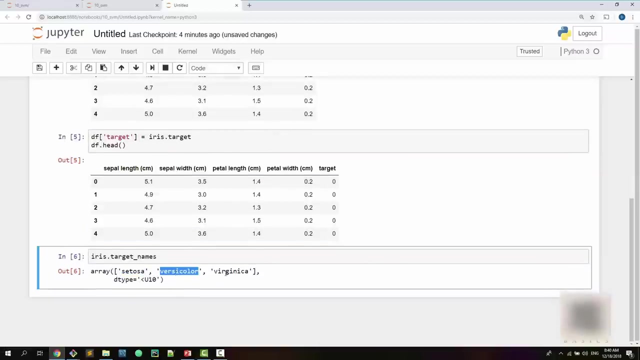 my data frame. so now I have my target, all right. so the target is the possible values. of target is zero, one and two. so what does zero, one, two means? so for that, if you do, I this dot target names. so zero index means setosa, one means versicolor three. 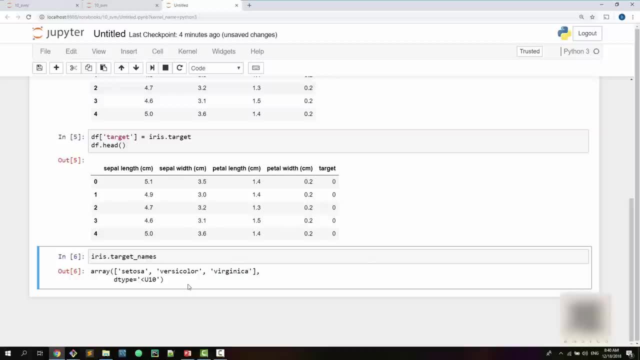 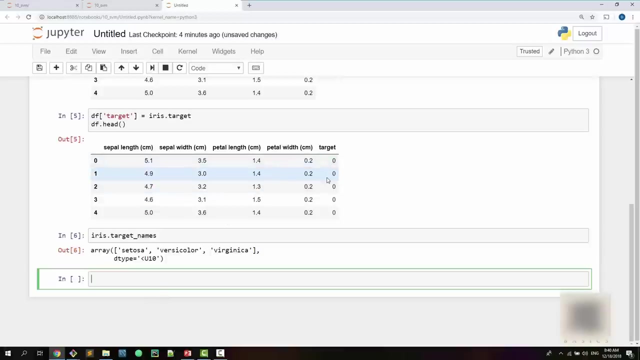 means virginica. so we have three type of iris flowers and the type is determined by these four features: sepal width and height. and length, the petal width and height. okay, all right, so now I want to. I want to do some exploration and see how many of my data 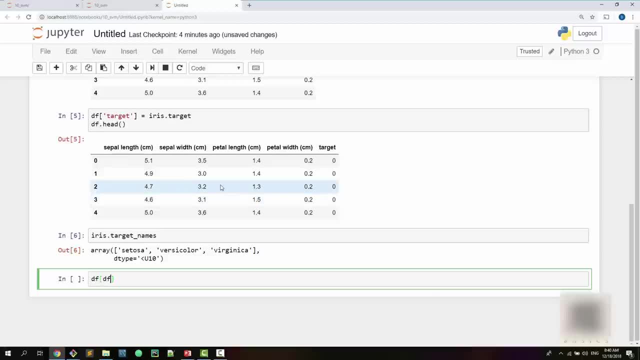 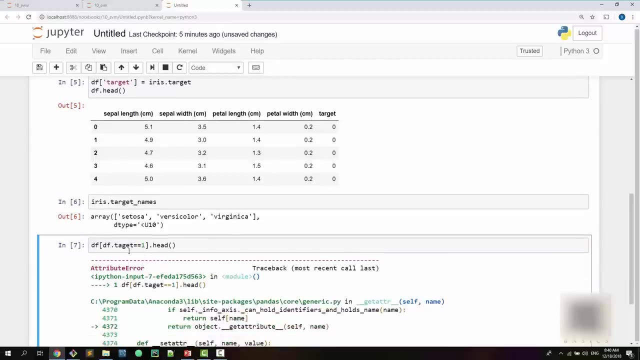 points have one in it. so what I'm going to do is I will say DF target equal to one. I want to see how many rows in my data frame has. uh, all right, I think I had a spelling mistake. so you can see from row number 15. 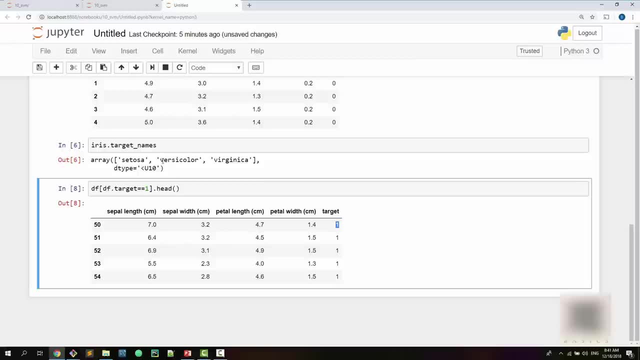 onwards. my target value is 1, which means it is versicolor. similarly, if i do 2, you will notice that it starts from 100 and my total data points is 150. so 0 to 50 is setosa, 50 to 100 is versicolor and 100 to 150 is virginica. let me add one more column. 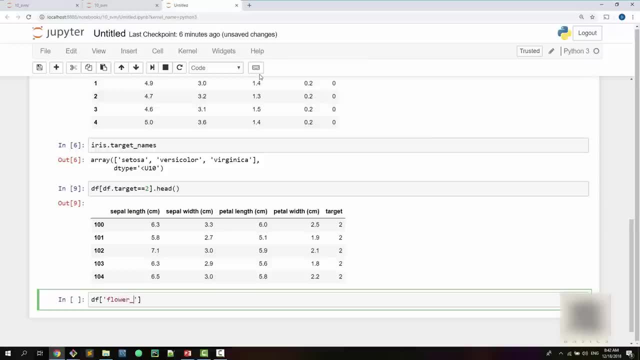 called flower name, so that it's clear. so flower name is equal to df dot target. so from one column you're trying to generate another column, and the way you do that in pandas is by using apply function, and here lambda is just a small function or a transformation that you can apply on target. 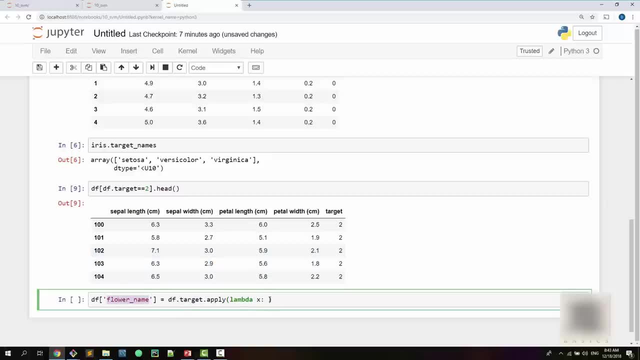 column and you can generate this new column called flower name. okay, so iris dot target names maybe. so for each value in my target column it will so that each value is x and it will return the index of the, the value in target names. so, for example, if it is two, so in this array zero, one, two is. 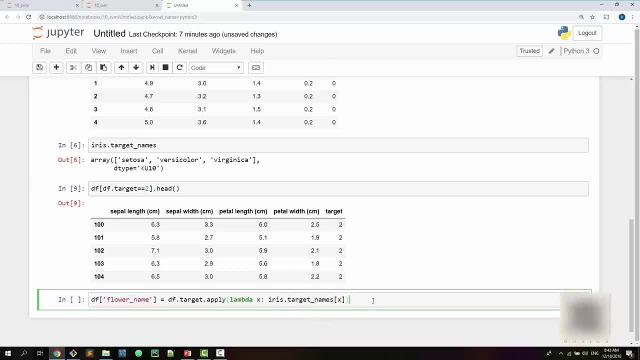 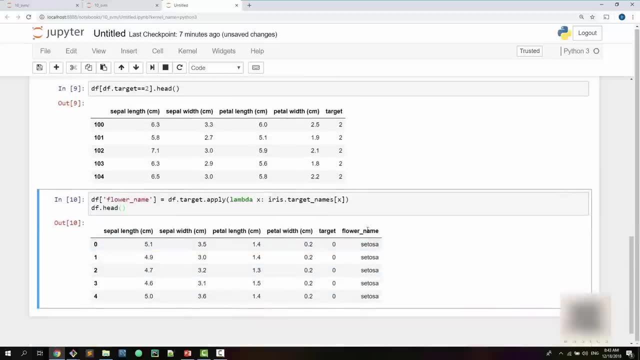 virginica. so virginica will be placed in flower name column and if you want to see it, you can see that now i have a new column called flower name. if you export this to csv file, it will be even more clear on how this data set looks. so 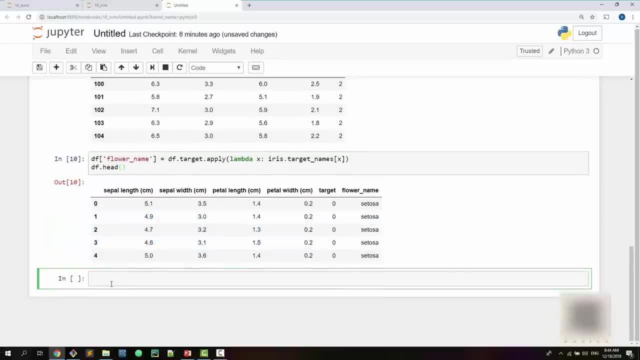 you can visualize it better. basically, now let's do some data visualization too, and you know that in order to do that, you have to, uh, use matplotlib. you can use some other libraries, such as bokeh, or there are a couple of libraries available for visualization. all right, so from mat. 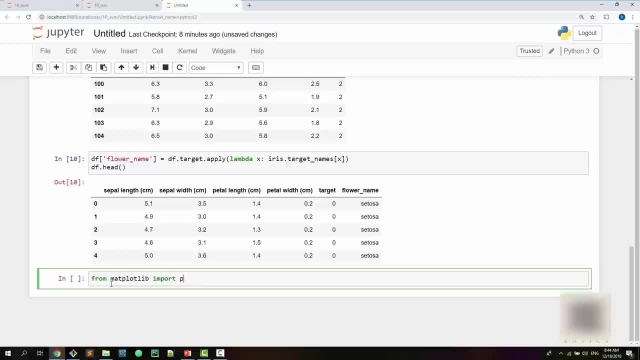 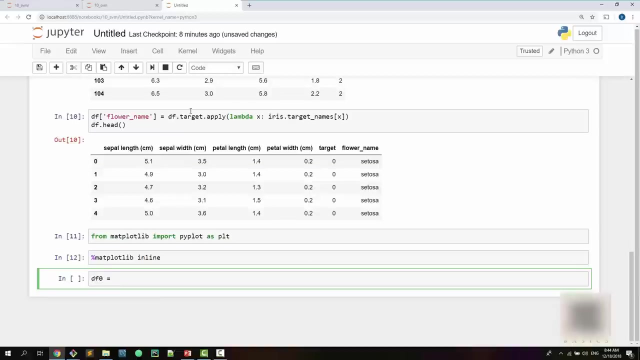 plot lib, import py plot s plt, and this is inline magic. this is a concept specific to jupyter notebook. all right, now let's first create three data frames. so i want to separate these three species into three separate data frames. okay, so how do you do that? df dot target is equal to zero is first data frame. 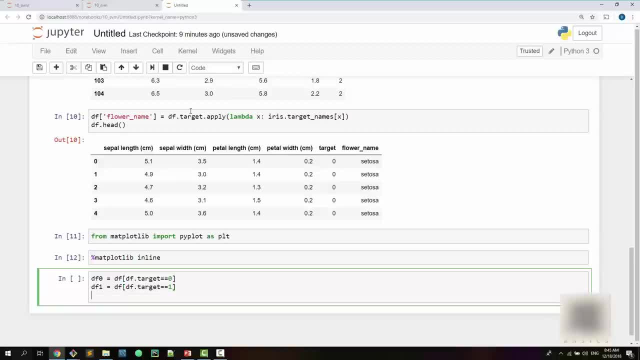 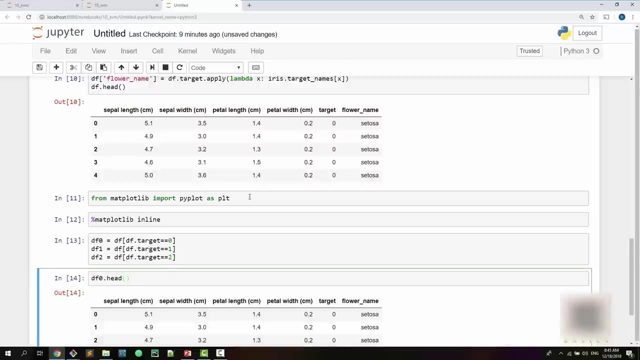 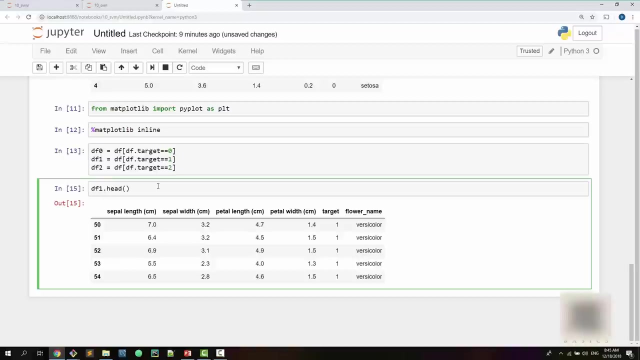 the second one is this. the third one is this: so now i have uh three different data frames, right, and if you want to look at those data frames, you realize that the first one is satosa, second one is versicolor, the third one is virginica. now let's uh draw a scatter plot. 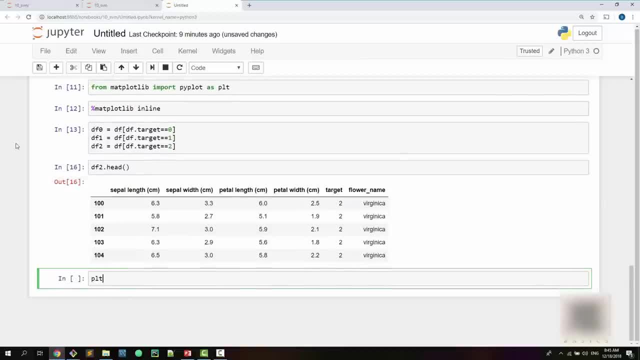 so you can do plt, dot, scatter and specify your x and y here, okay, so what is your x and y? so i'm going to plot the first two flowers. so df 0 and it's a 2d plot, so i will only use these two features. okay, so let's do this. 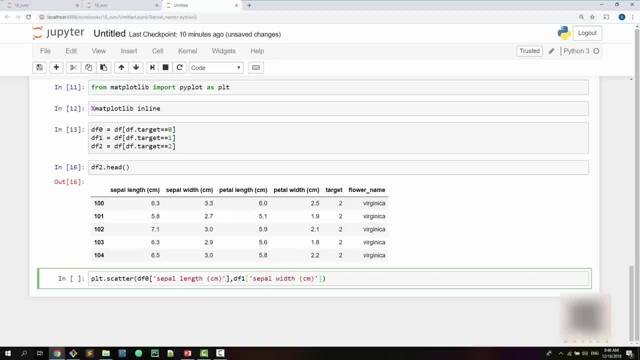 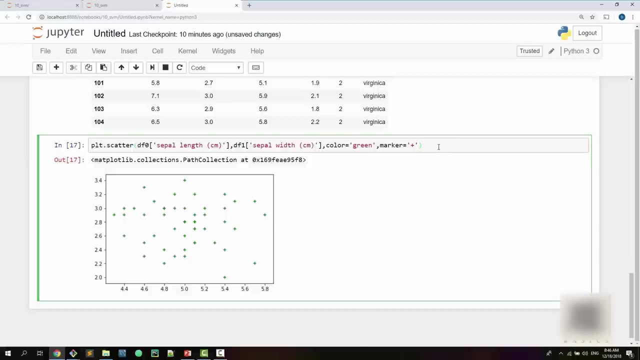 you can specify color and marker. okay. so let's say, my marker is this, so my scatter plot looks like this. okay, now i will do the same thing. actually, i made a mistake. i should have done dm, so i will use it back to my data frame right now. 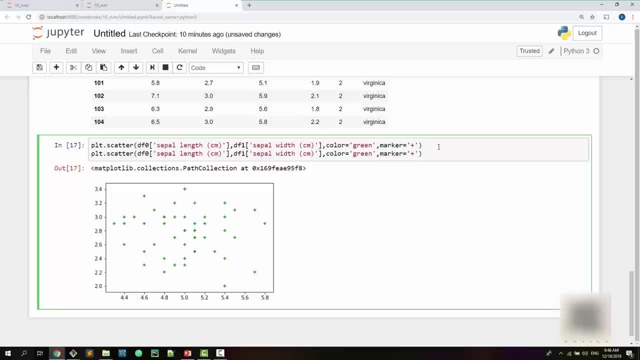 let's now do the same thing. okay, so i have two decals, i have a full data frame, so i will choose it as that. and also i have two decals for the title model, so let's do it then. 0 actually. so df0 is a sample width and df1, and let's say, this color is blue, so you can see that. 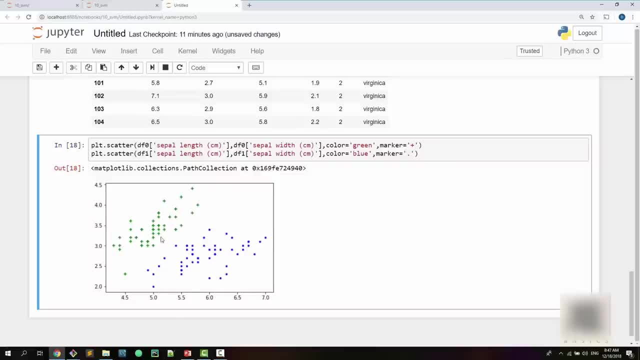 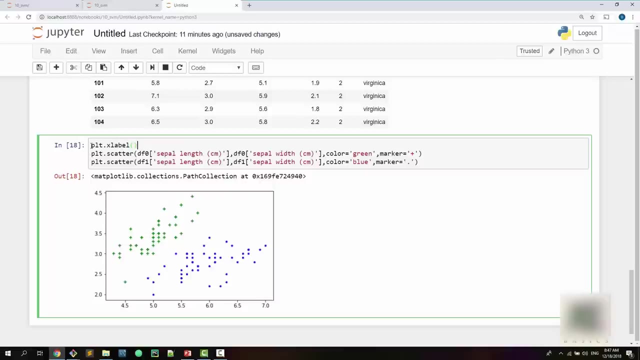 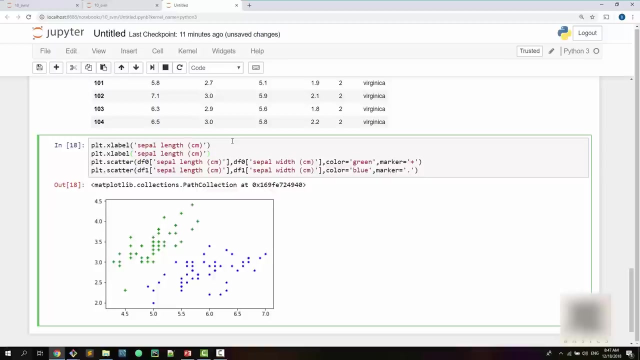 there is a clear classification. so if I use my SVN or SVM algorithm here, it will probably draw a boundary like this. all right, you can also. just to make this plot clear, you can specify X label and Y label also. so what is my X label? X label is sepal length and Y label is my width. 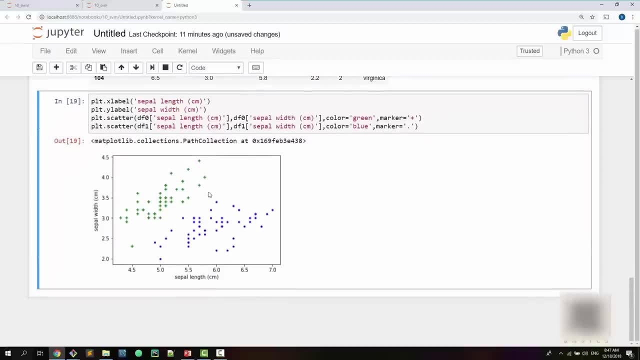 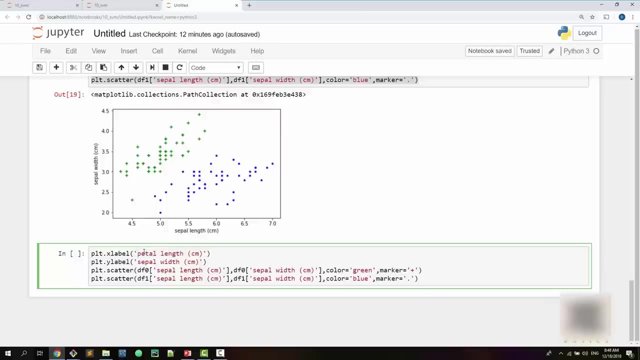 you know when you're looking at the chart now, it's very clear. all right, let's plot better length and petal width also. okay, so I'll just copy paste this guy here. all you need to do is replace Apple with petal, and this is just plotting two more features, and you can see that this has even clear. 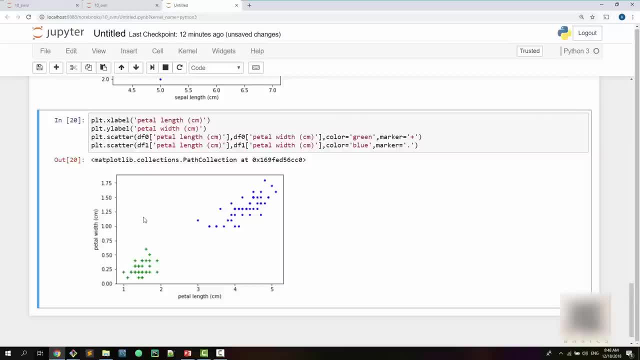 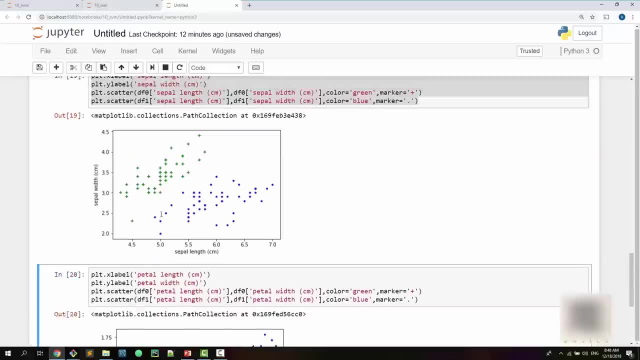 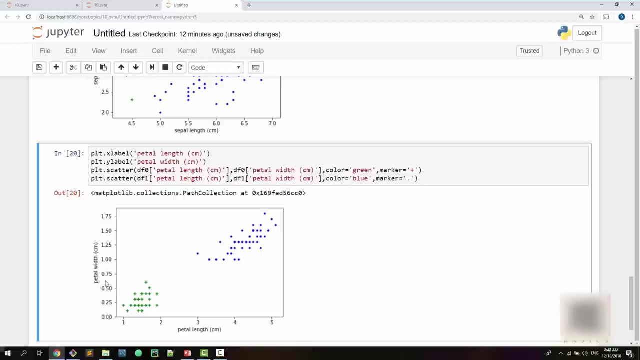 classification. so looks like our SVM is going to perform really well because it will be able to easily draw very nice and clear boundary between these data points. now here I have plotted only two features each on on these scatter plots, actually, when we train our algorithm we are going to use 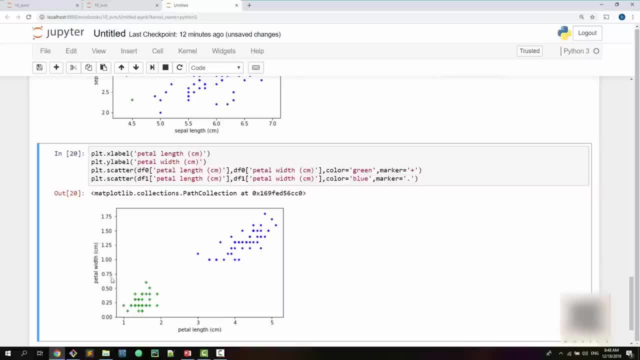 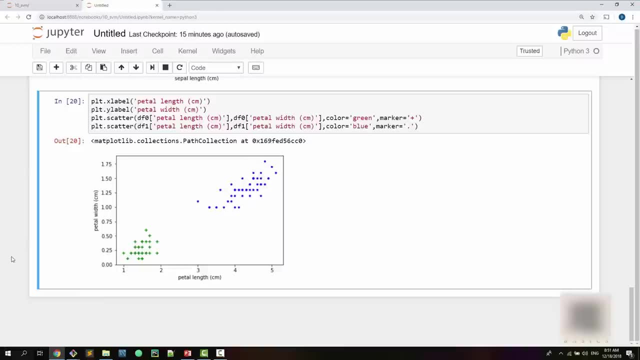 all four features and the classification will also be between all three species. now let's train our model using sk learn right. so the first step is, as usual, use train test split to split your data set into training and test data set. remember, you don't want to test your model on the same data set that you have performed. 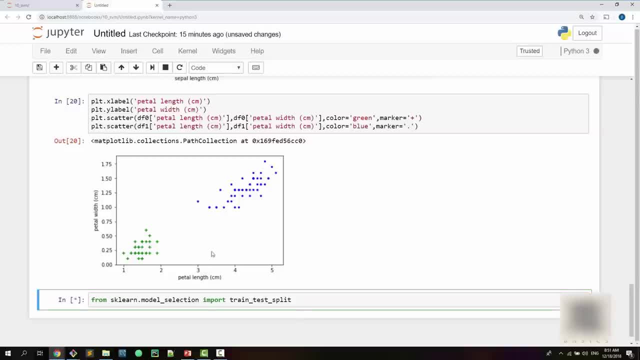 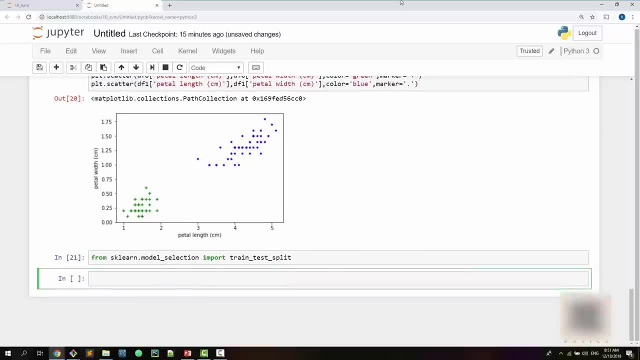 training on because it might be biased. okay, so let us do this. our DF data frame has target column also, so I want to remove those first. all right, and the way you remove them is: you want to say I want to drop certain columns from my data frame, and which are the which are: 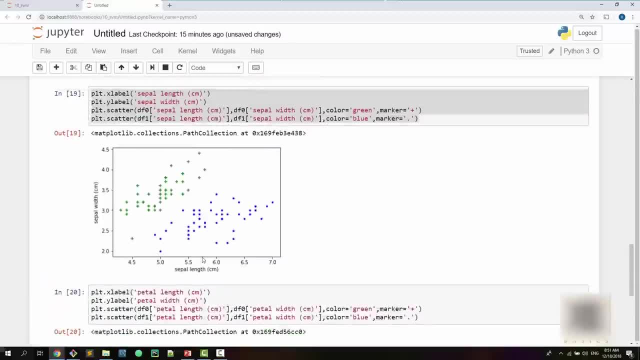 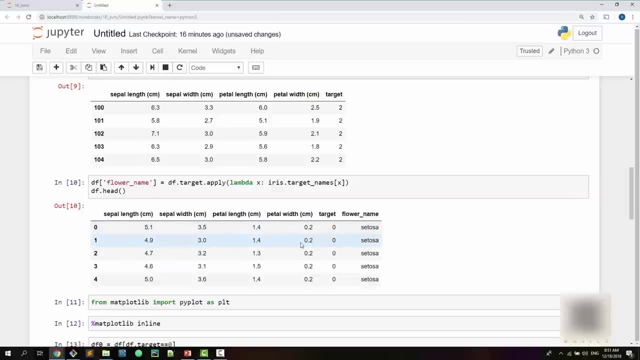 the columns that you want to drop. okay, so let's look at our data frame. our data frame has all these. okay, out of this, first four columns are your features that you want to use for training your model. second two columns are your target columns. okay, so I want to drop target and flower name. 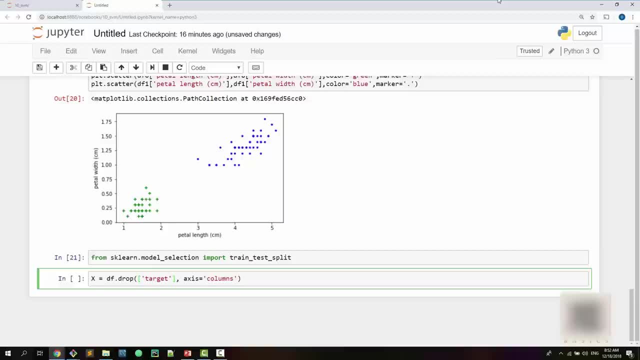 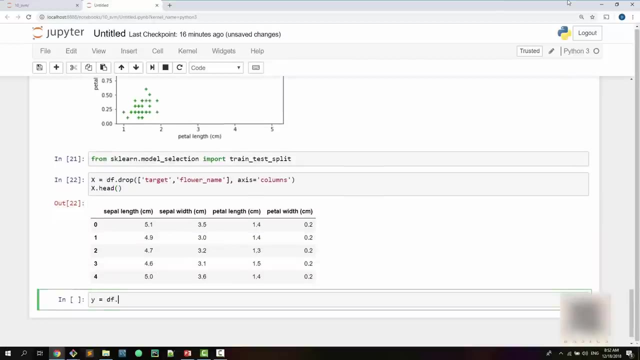 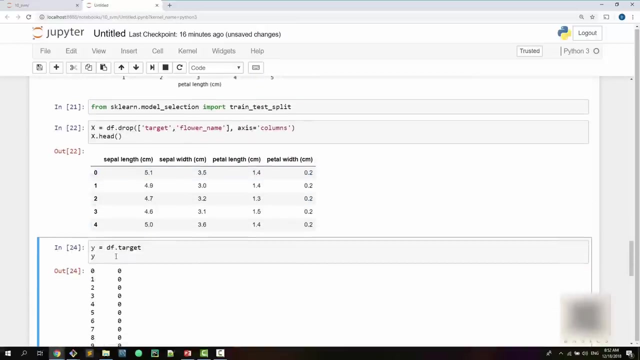 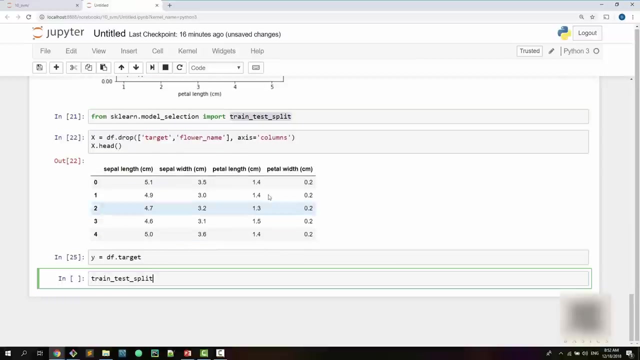 perfect, and my Y will be just dftarget, okay. so if you look at Y, it's gonna be your usual numbers between and two. okay, so now let's use train this split: X and Y, your test size. let's say I want to use 20 percent of my samples as a test and 80 as a training. all right. so X- train, the output of 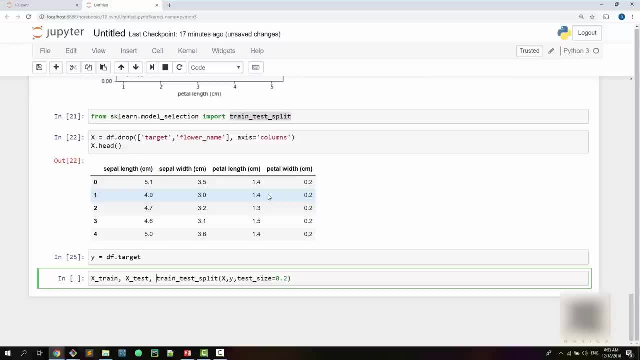 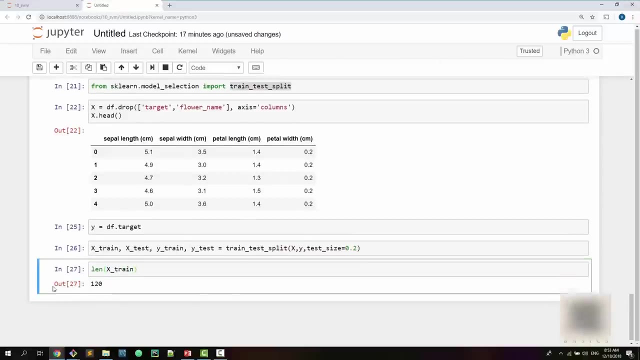 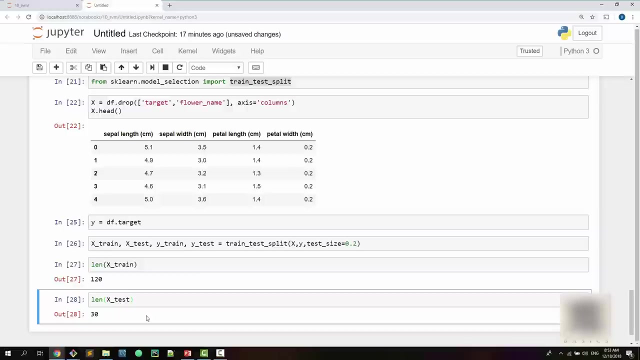 this train test split method is X train, X test, Y train, Y test, and if you look at the length of your X train and X test, you will notice that, uh, this is thought 20 percent of your 150 samples. right, so it looks good now. now let's from sk learn. 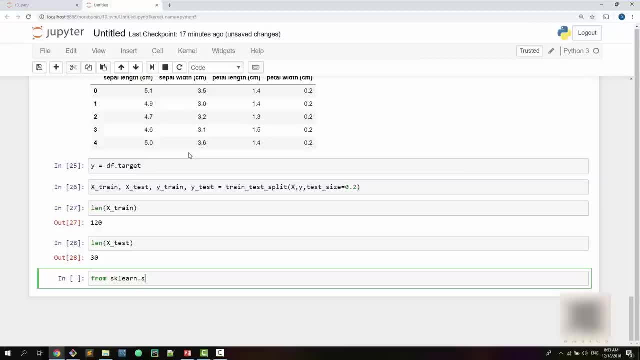 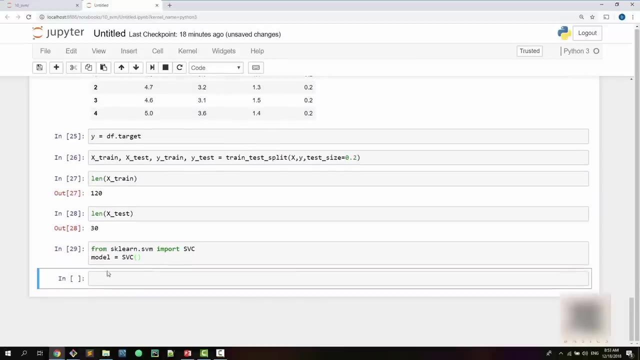 dot SVM, import SVC, so the classifier is SVC basically, and this is how you create SVM classifier and, as usual, you can call fit method to train your model. okay, I'm going to use extreme Y train, so my model is strain. you will notice some parameters here, such as C, if you remember from. 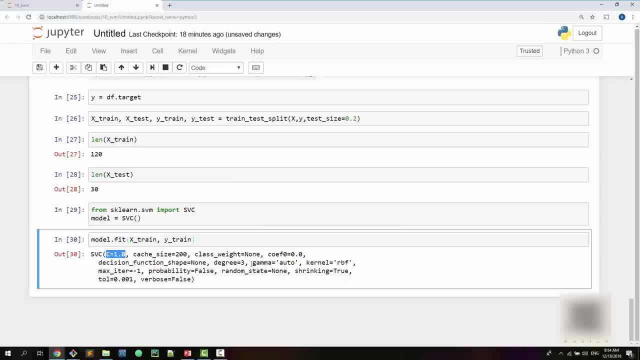 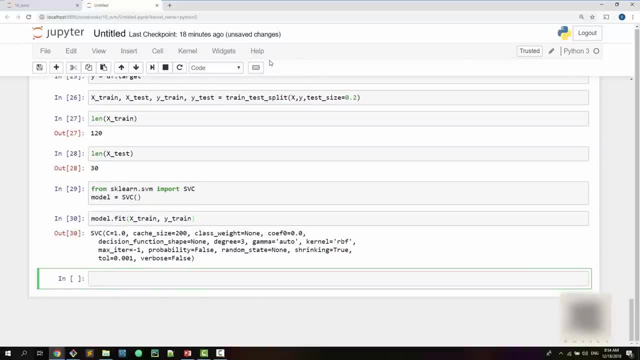 the presentation earlier. this is a regularization parameter. you have Gamma also and you have kernel. okay, all right. now let's look at the accuracy of our model. you can call score method, and now this time I'm going to use x taste and Y taste. So my model is train and I am performing the accuracy of this model by supplying this X. 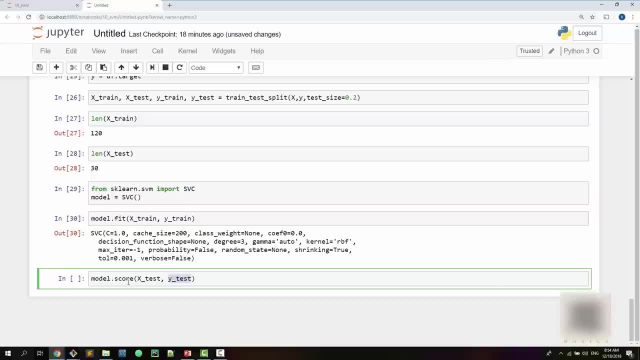 test and Y test. What the score method is going to do is it will take X test, It will predict the values, So it will be called like Y predicted and it will compare Y predicted with Y test to measure how accurate the model is. 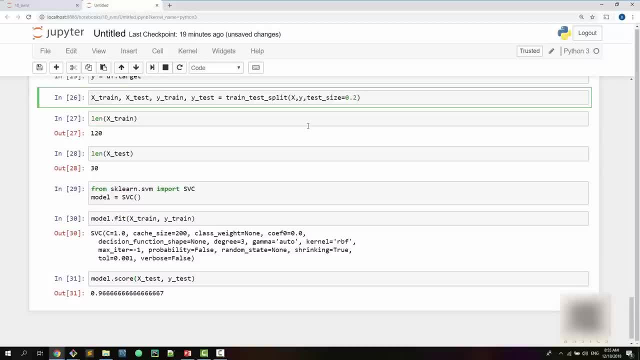 And you can see that it is 0.96.. If you execute this again, your X train and X test changes. you know the sample changes, So I want to not train it on a different set of samples. So again it's like 0.96.. 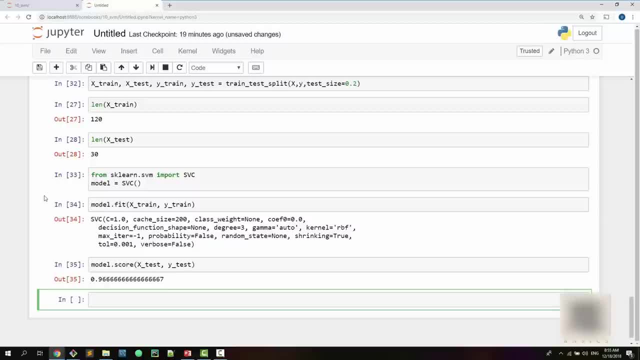 You can now use the separate parameters. For example here: by default, C is 1.0.. So what if I modify the C parameter? Let's say you do, C is equal to 10.. And on the same data set, if you train it. 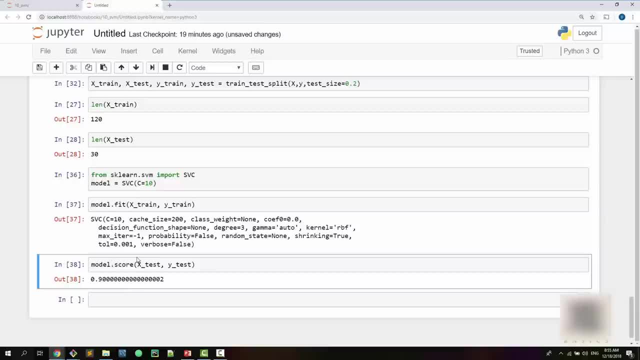 See, increasing regularization is actually decreasing my score. So you can use these parameters to tune your model, and you can do this on like a couple of data sets, using cross validation techniques, and you can figure out what parameters are best suited for your given problem. 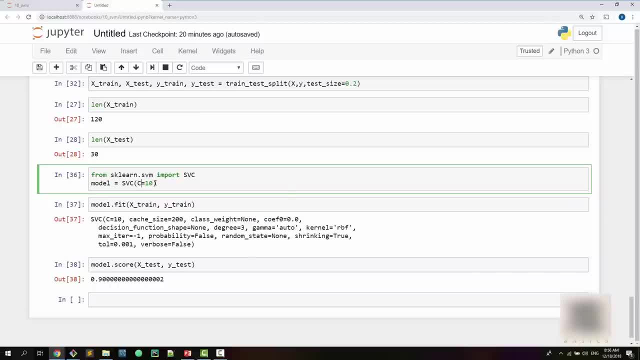 Right, You can use even gamma also. So gamma is- Let's see, if I use gamma, Gamma is equal to one. What happens? OK, I get the same score. Gamma is equal to 10.. Again, the same score. 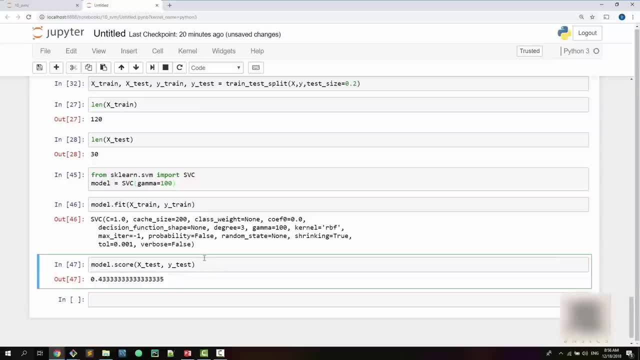 So it looks like this is not making much difference. Also, gamma 100 is going to make the model performance worse. All right, You can also use kernel. So by default, the kernel was RBF. Let's use linear. Now how do you know which kernel to pass here? 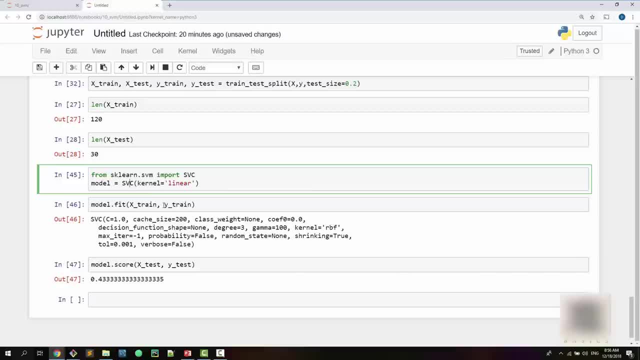 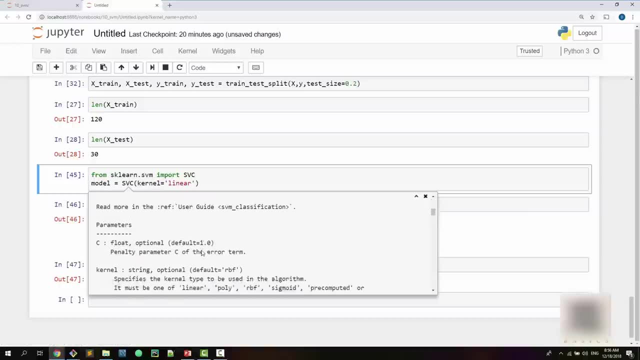 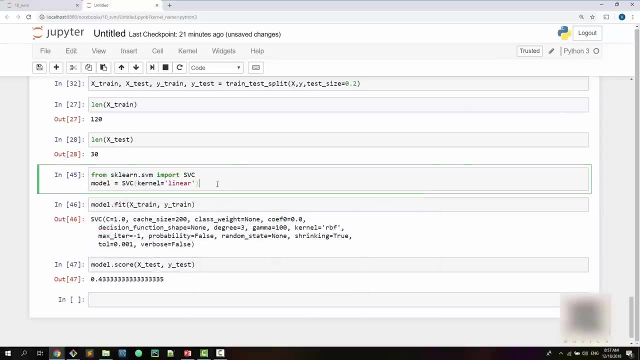 Right. So if you use shift tab, it will show the help from the SQL and API and you can say: these are the possible kernels I have available to use. All right, So let's do linear, And with linear also you are getting a very high accuracy score.